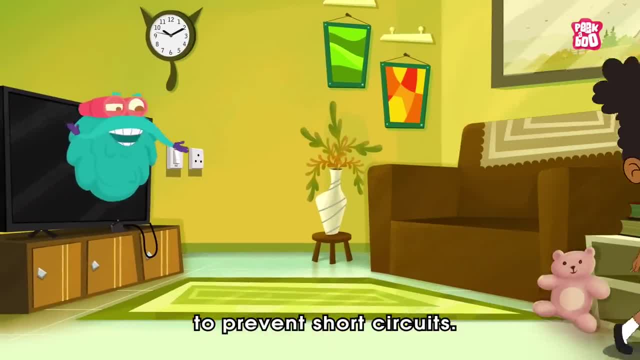 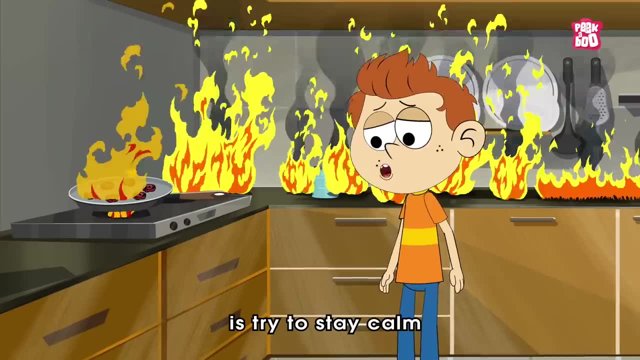 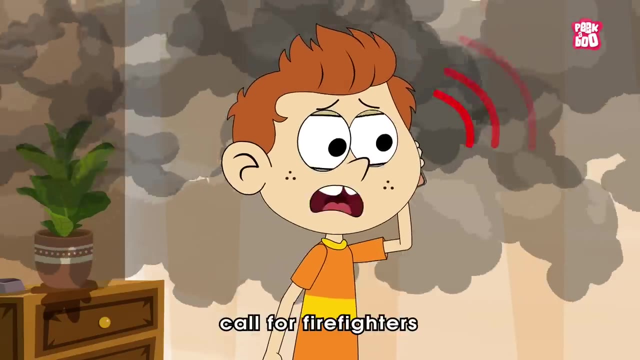 when you're not using them to prevent short circuits, But in case a fire does break out, the first thing you should do is try to stay calm and not panic, so that you can think clearly, Then immediately call for firefighters and alert everyone in the house or school. 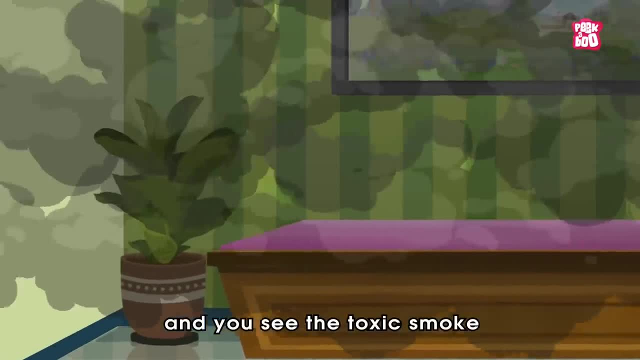 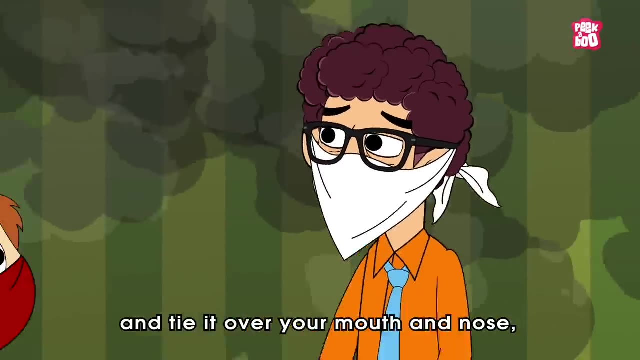 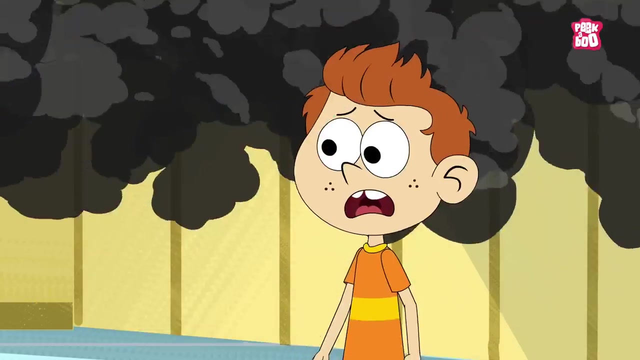 And if there is no easy escape route and you see the toxic smoke filling up the space, then quickly soak a cloth in water and tie it over your mouth and nose, as breathing in too much smoke can cause you to pass out, Also, as this smoke tends to rise up. 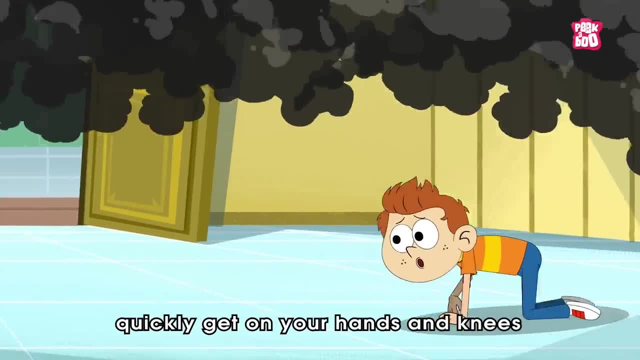 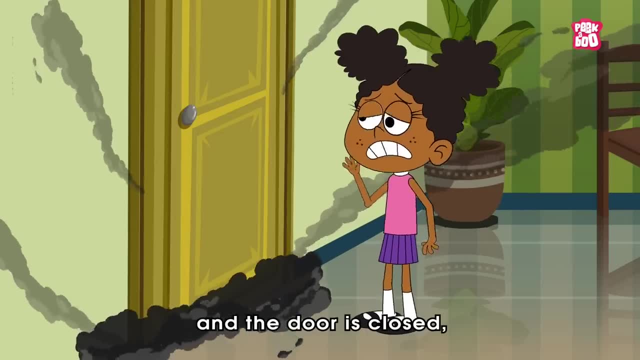 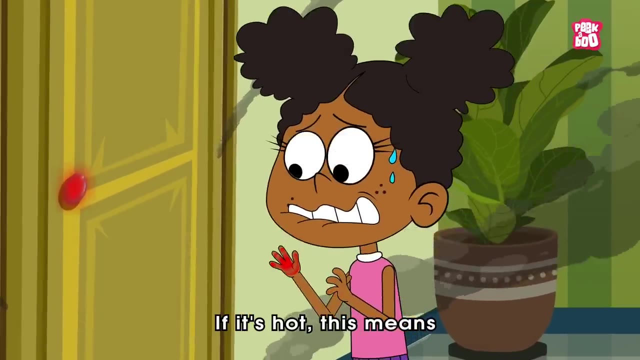 to give yourself some extra time. quickly get on your hands and knees and crawl towards the nearest exit And if you're in a room and the door is closed, check to see if it's hot before opening it. If it's hot, this means there's a fire on the other side. 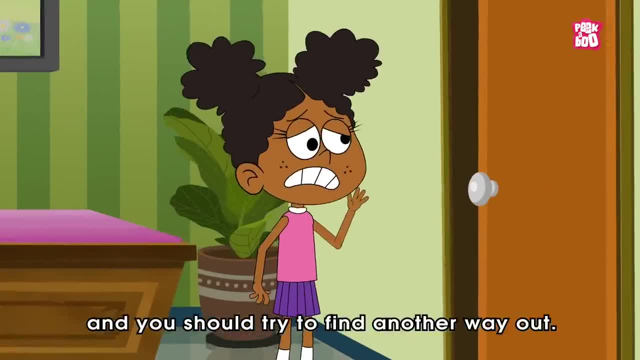 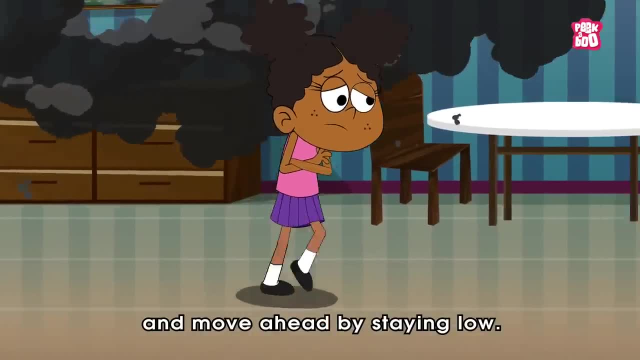 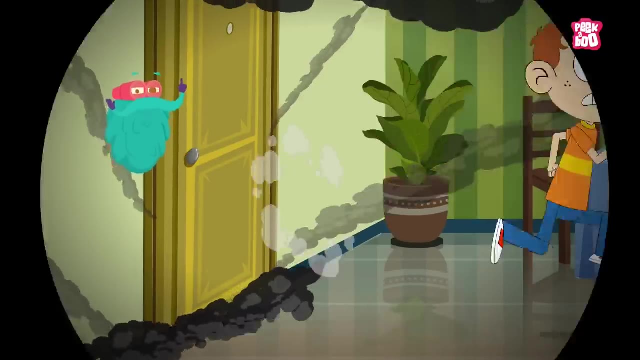 and you should try to find another way out. If the door is cool, then open it slowly and check for smoke or flames and move ahead by staying low, And if you're trapped in a room and can't get out, try to seal the room off as much as possible. 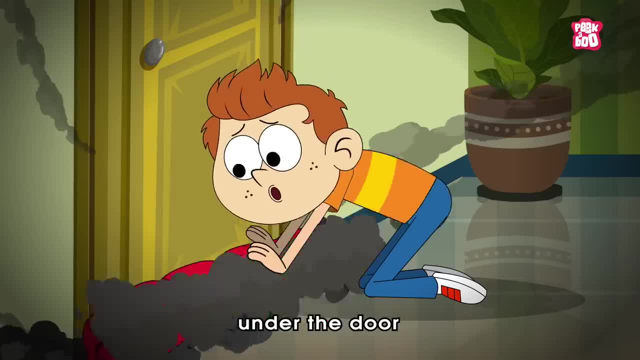 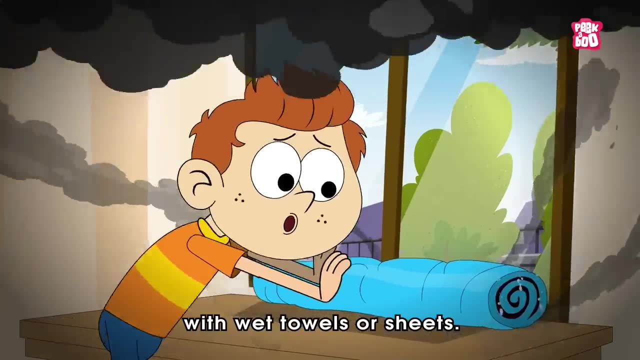 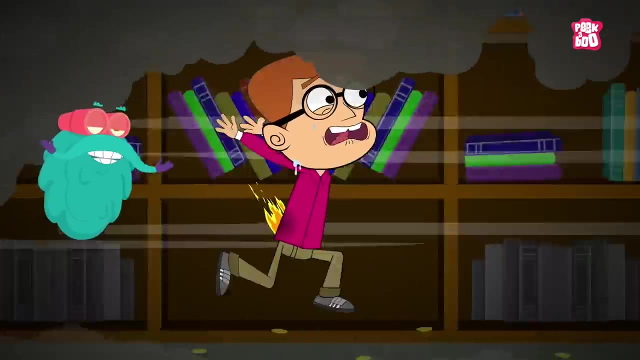 Stuff clothes or towels under the door to stop smoke from coming in and seal any gaps around the window with wet towels or sheets. And by any chance, someone's clothes happen to catch fire, then use a safety technique called Stop, Drop and Roll. 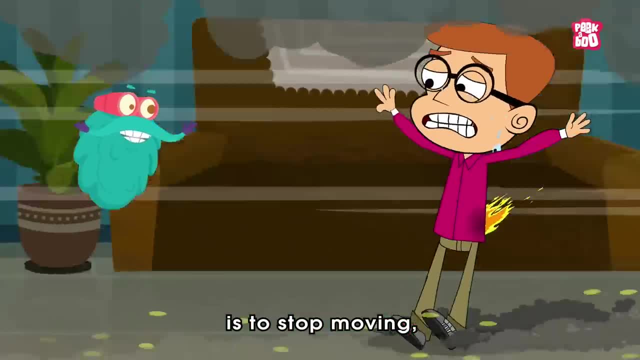 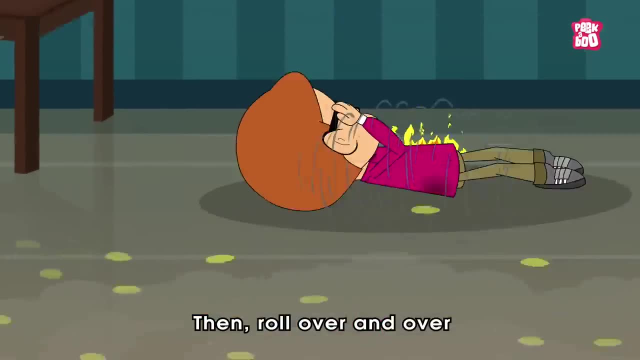 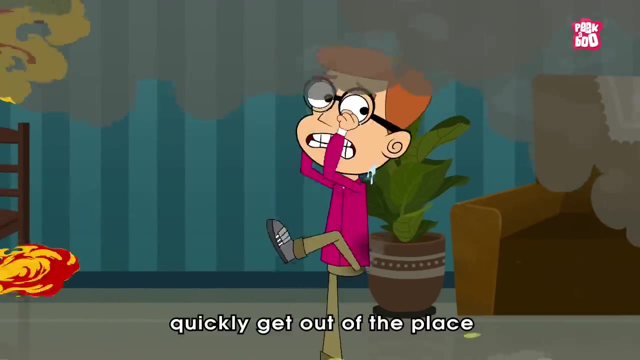 According to which the first thing to do is to stop moving, drop to the ground and cover your face with your hands, Then roll over and over until the flames are extinguished and, once you are out of the toxic smoke zone, quickly get out of the place.